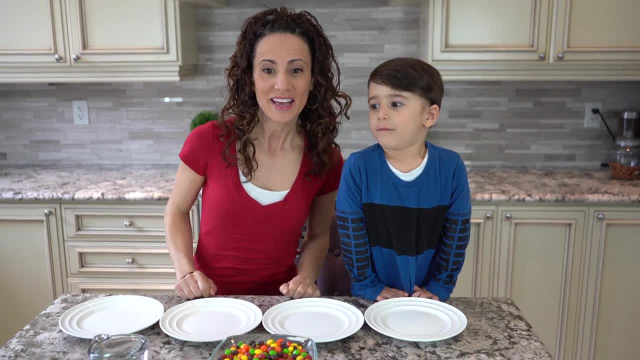 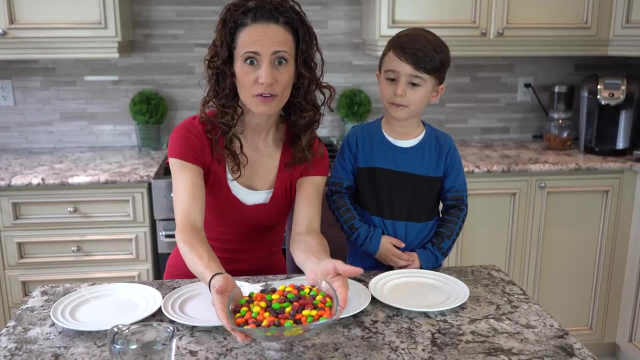 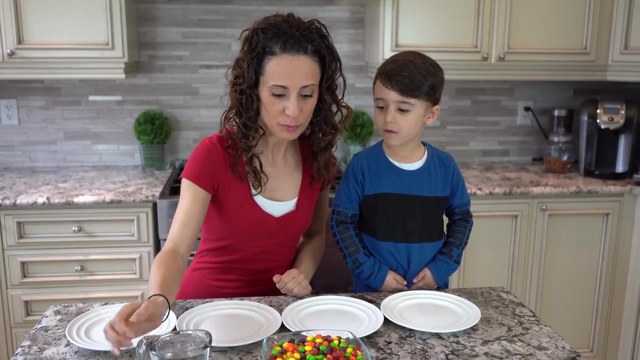 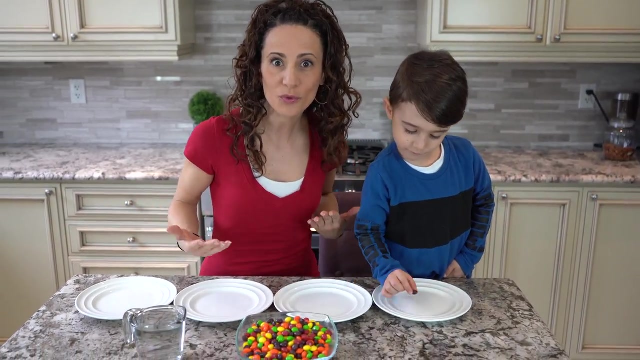 Our first experiment today is a Skittles experiment. Now, what you need is very easy: Just a few plates, some very colorful and tasty Skittles and some warm water. So what we're going to do is we're going to put the Skittles inside the plate- and you can do them in all different ways, and we're going to see what happens when we pour the warm water in. Okay, Mateo, you start Go. What are you doing? You're putting Skittles. 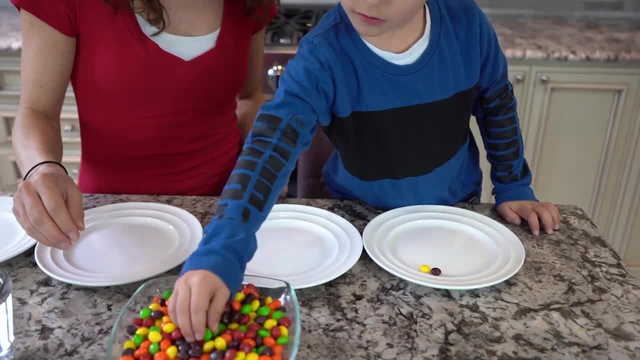 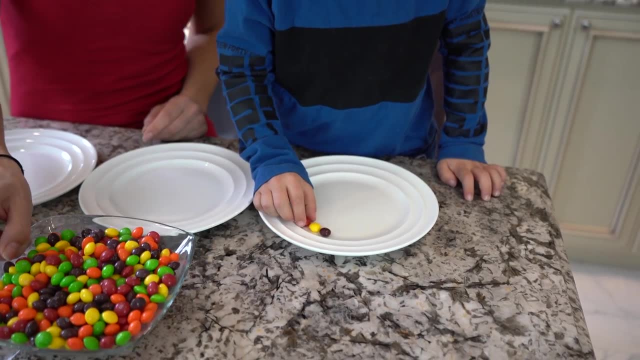 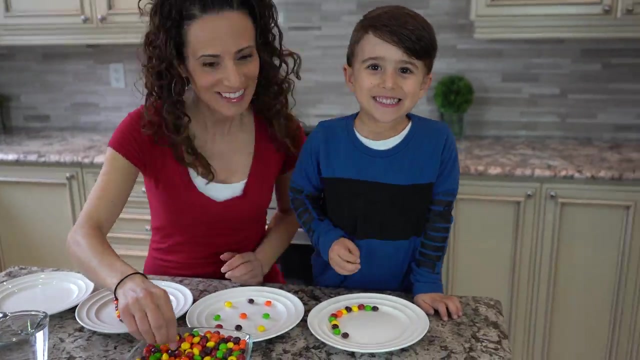 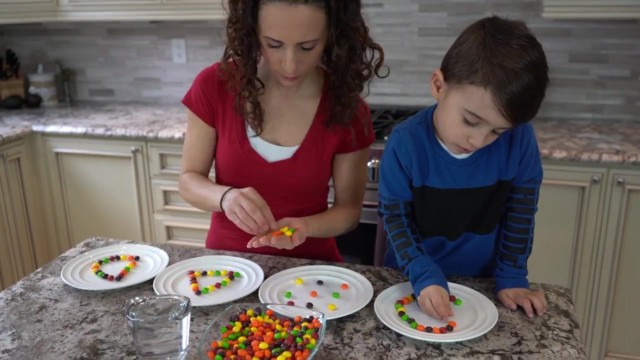 Skittles, all different colors. right, Yeah, Nice, Are you making a rainbow with those? Yeah, Okay, Pretty cool. Now Mateo's doing these. I'm going to work on this plate. Now we put all the Skittles in the plates and they're all different Mateo did here. What did we do here? 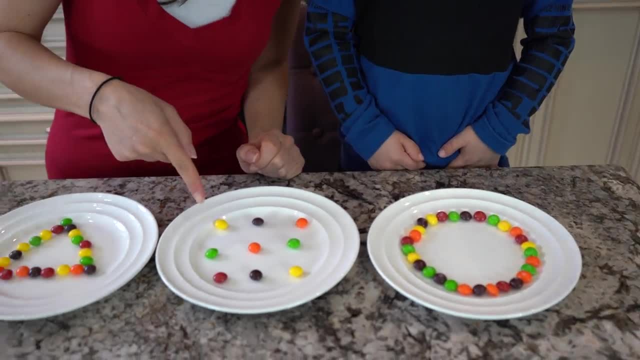 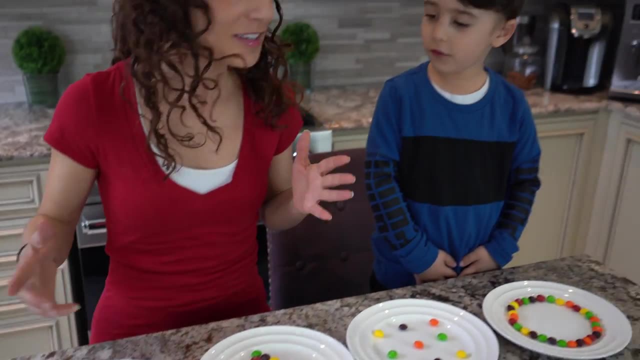 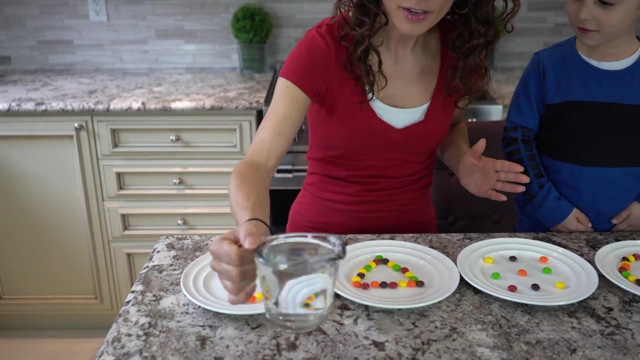 A circle With a nice rainbow I did here. I spread them all out. This one, I did a triangle And a D And a D for D. So we're going to pour the warm water in and we're going to see what happens. I'm very curious to see how they all come out. Okay, Let's pour some warm water in the middle of all of them. Here we go. 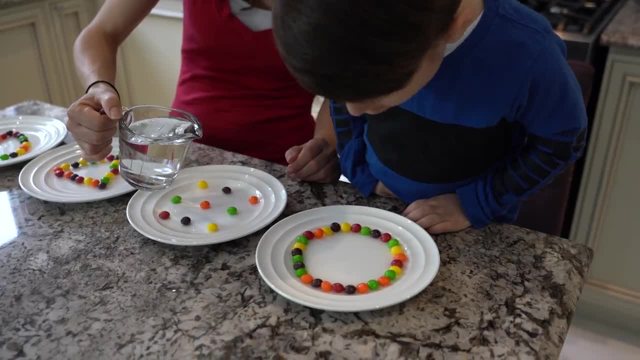 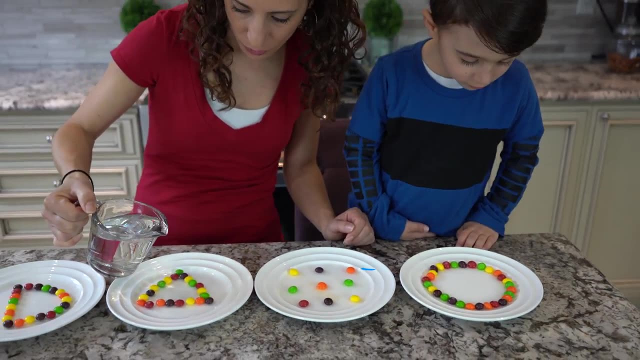 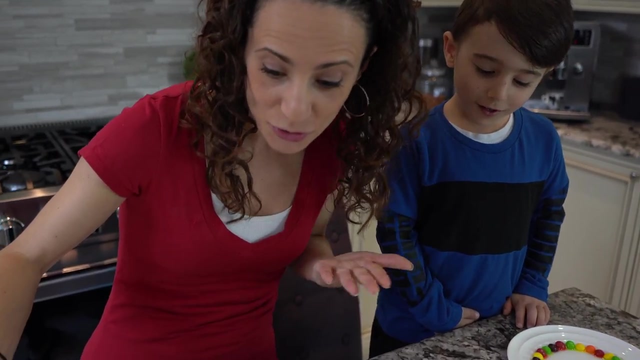 Whoa, Look at that. Yeah, Now we're going to wait and we're going to see how all This is how they come out now Ready. We're going to have to give it some time, though, And because they're all different shapes- Whoa, Look at these ones. Yeah, They're all different shapes. It's coming out. They're all going to look different. 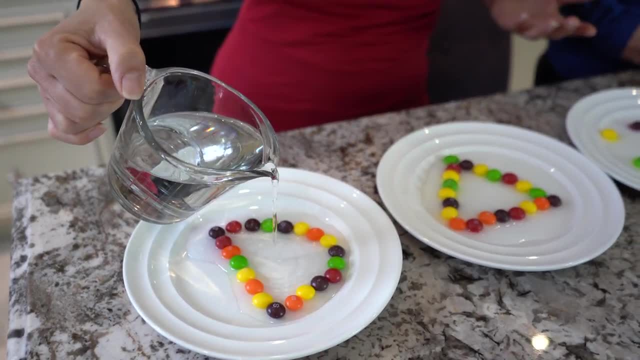 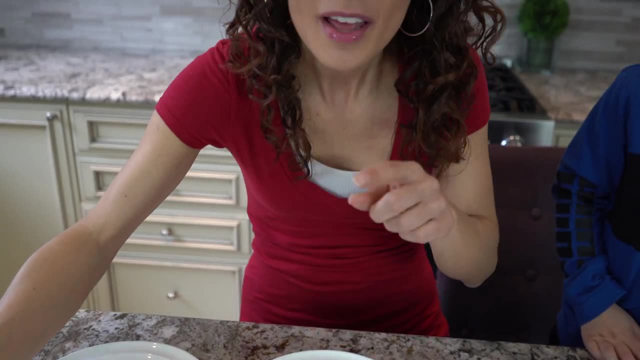 Which is awesome. Whoa, Look at it. Yeah, Okay, Let's see, Okay, Let's see what happens. Ooh, Look, Come see, This one is already starting to melt. Look, Wow, That's pretty cool, Mateo, Cool, All the warm water. 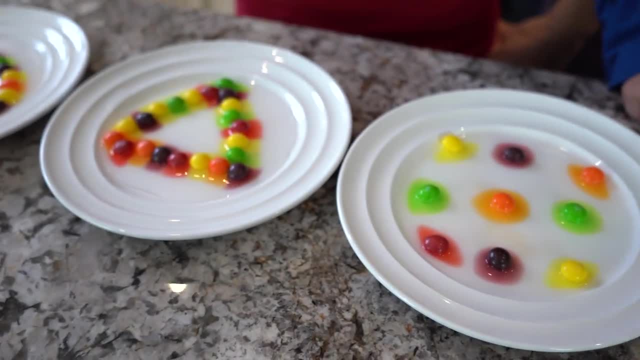 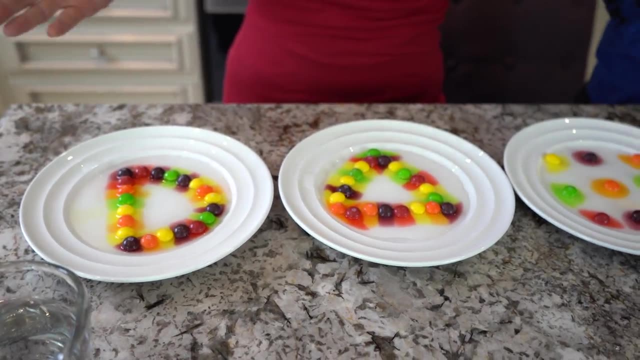 Even this one and this one and that one. They're all melting. Yeah, All the warm water is melting the candy from the outside of it. Wow, It's making a cool design. So you guys can do them all different ways. So depending on where you put the candies, it's always going to look different. 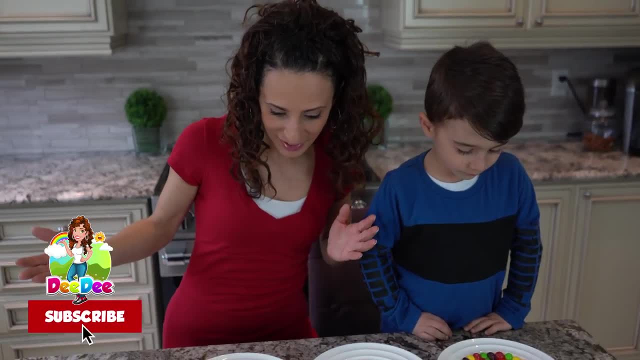 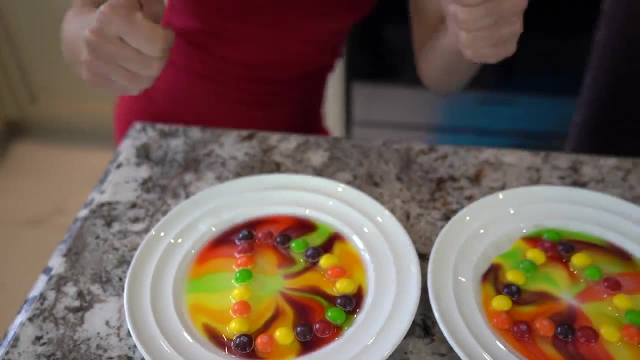 And even depending on what color candy you put, Pretty fun, I love it. Music For our second experiment: we are doing a drawing. Music For our second experiment: we are doing a drawing. Music For our second experiment: we are doing a drawing. 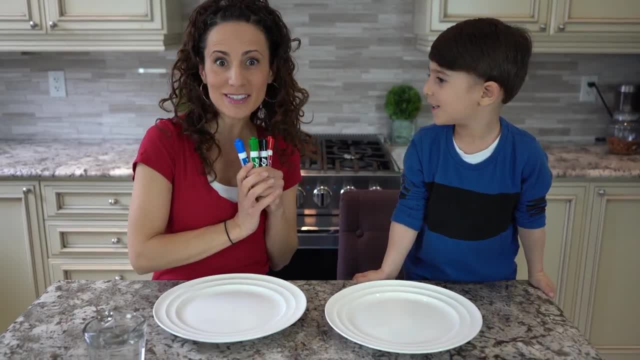 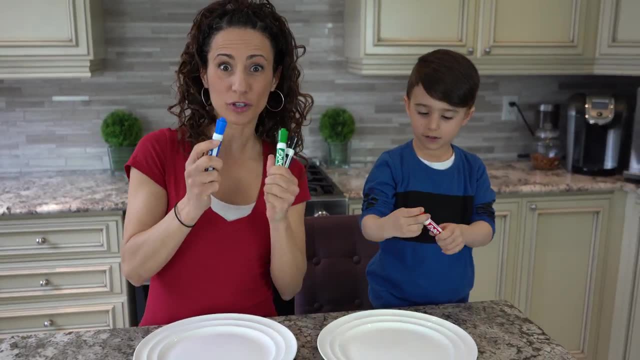 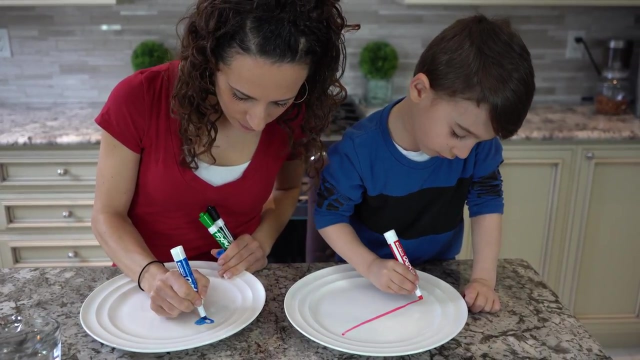 dry erase marker flow. are you ready to write on some plates? yeah, yeah, okay, what color do you want to pick? um, this one, the red. okay, i'm gonna pick all different colors. wow, okay, i'm gonna do with stripe, with with zigzags, oh cool, okay, i'm gonna do some hearts on mine. 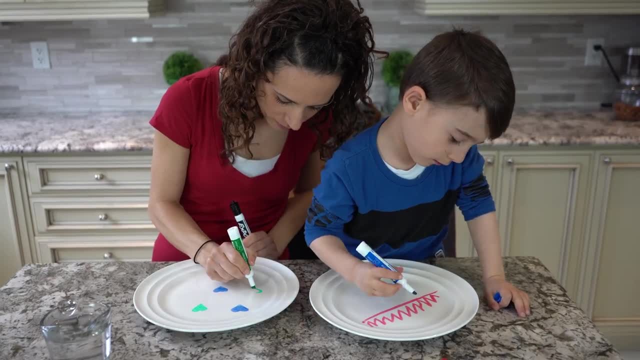 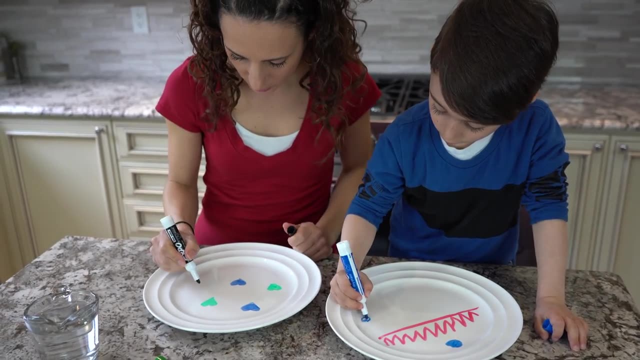 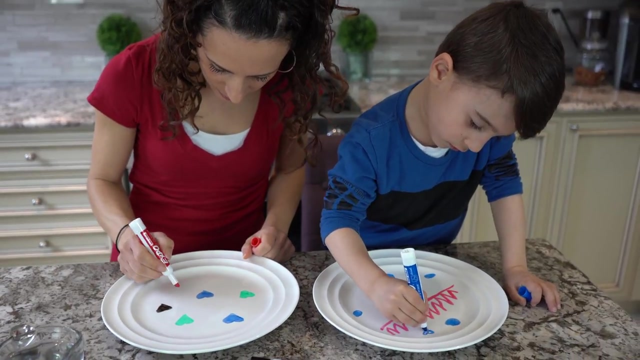 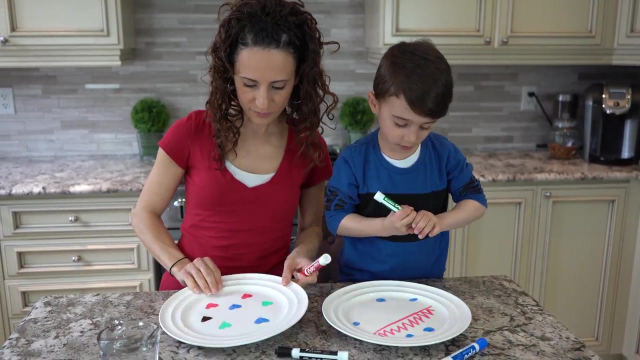 okay, i'm gonna do um a circle here. nice, oh, that's a good idea. the circles are good. another one here, another one here. good idea here. okay, okay, are you finished your design? nope, not yet. not yet mine's finished. look what i have. i need a. i need i did all different color hearts on mine. i need a cross. 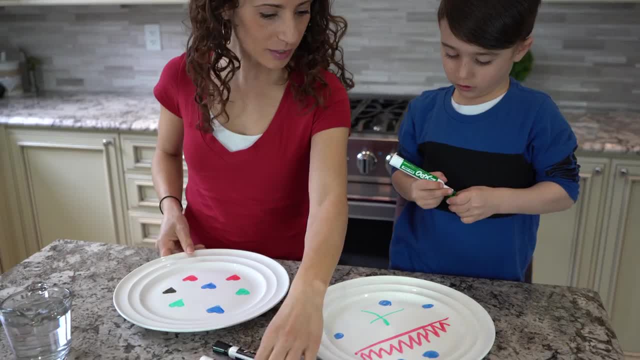 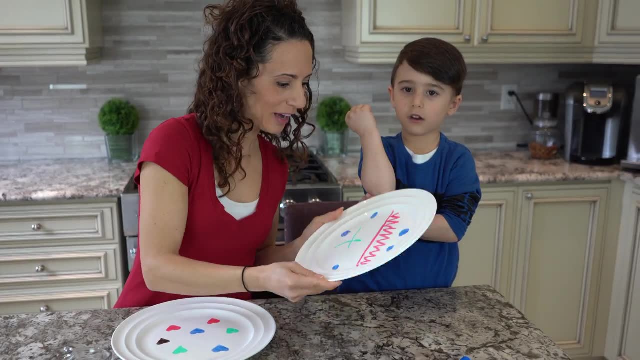 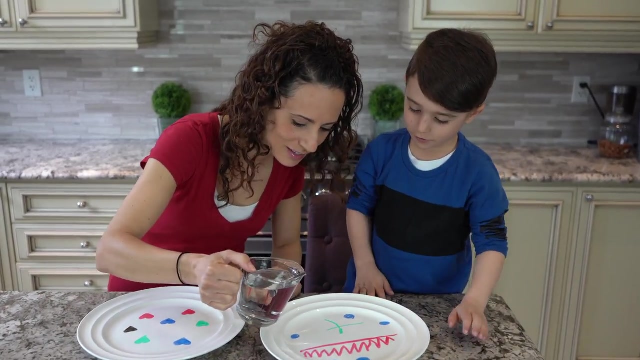 okay, okay, you ready, done, done. you want to show everyone that's a monster, that's a monster. look at that. that's pretty cool, okay. so now? what do we do? now, we drew the picture. what do we do? we water, we pour water, and let's see what happens. see how you're. i think the monster's gonna break. 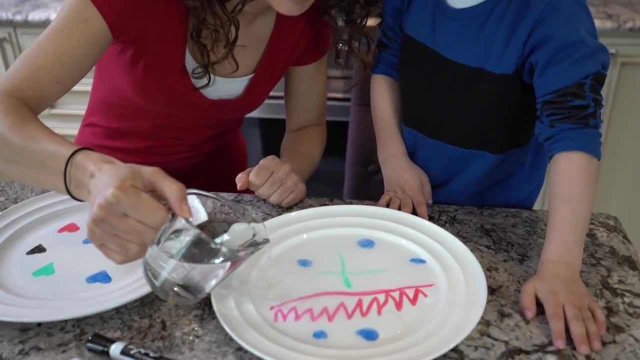 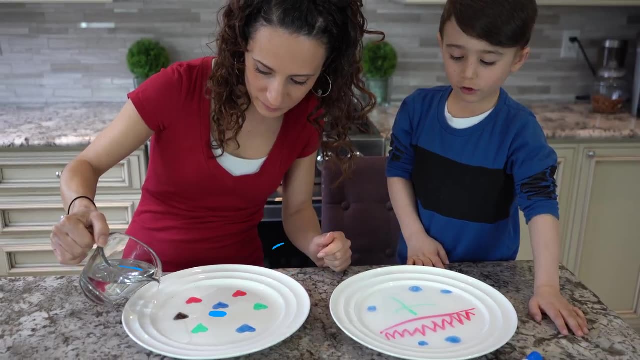 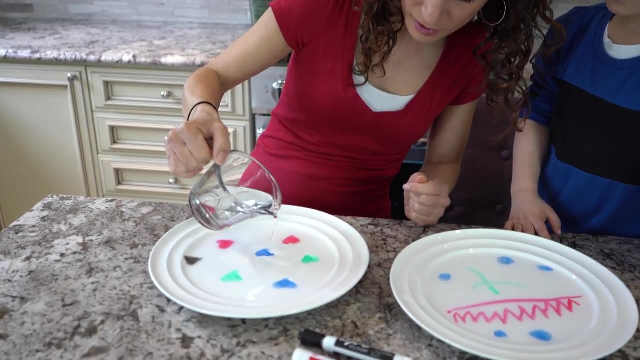 off. you think, oh, oh, my goodness, look at so they're all floating. look, they came off the plate. so so the monster is still alive, is he? yeah, look at mine. look at my hearts. they're coming off. that's cool. the black one goes now. yeah, look, it came off now. okay, look at mine. they're almost. 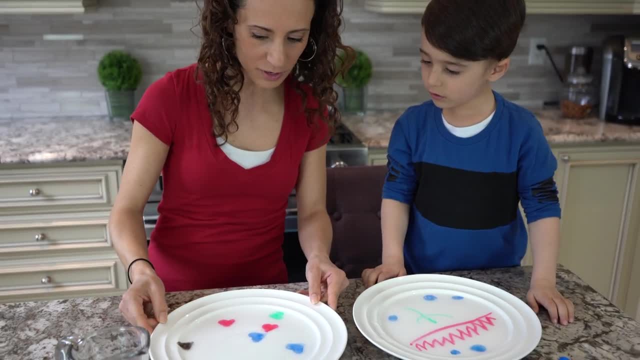 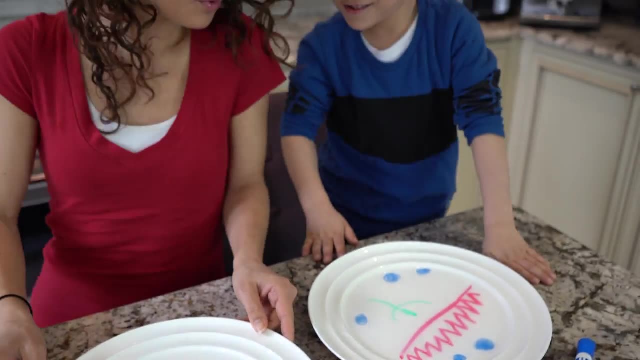 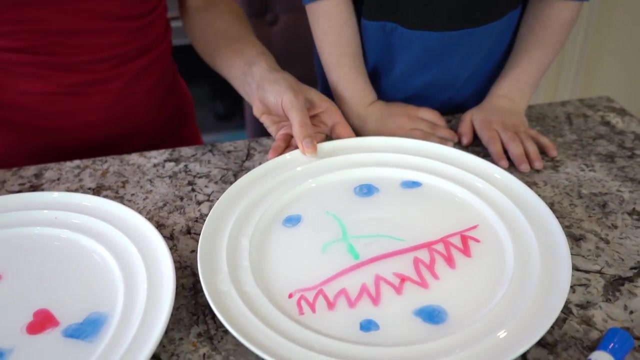 all off hold on a second. oh look, mine are all floating, look at me, look at them. mine are not floating, mine are like dancing. how do we dance? how do they dance? how are they dancing? dances, okay, is yours floating? yep, oh, yours is dancing too. yours is cool. oh, the chief is breaking. oh man, okay, are you ready to do something cool? 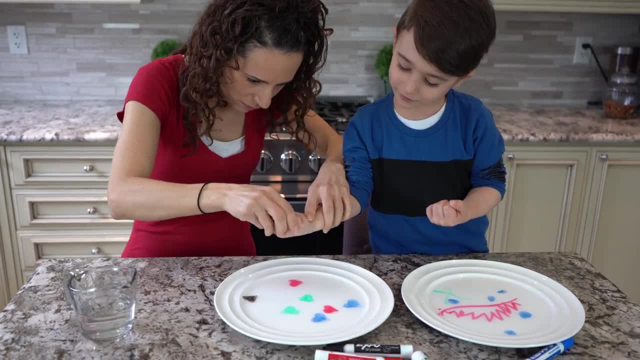 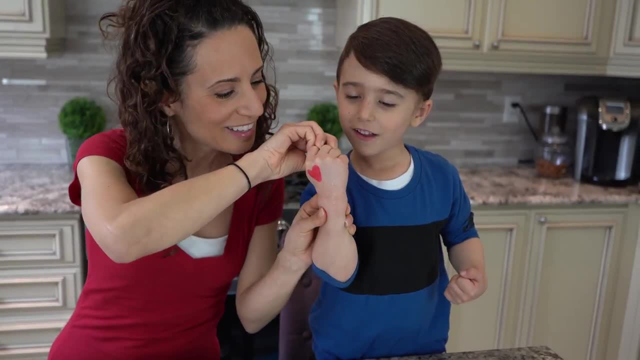 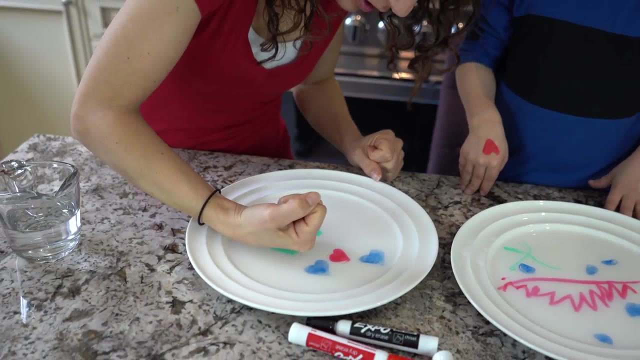 yeah, put your hand up ready and let's put it on the right one. what happened? oh, it's stuck, that's cool, okay, that's cool, okay, i'm gonna do one. which color? i'm gonna do the green one, see if i get mine on. mine is so cool, okay, did mine stick. mine's stuck too. 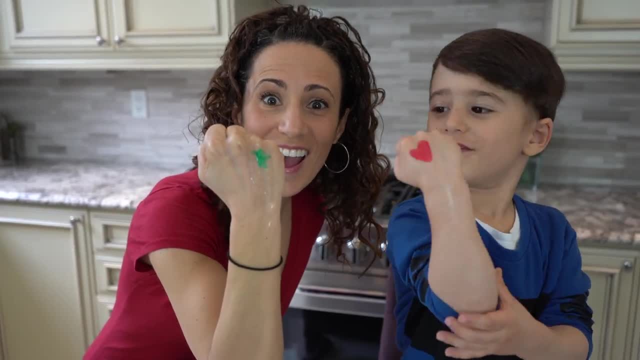 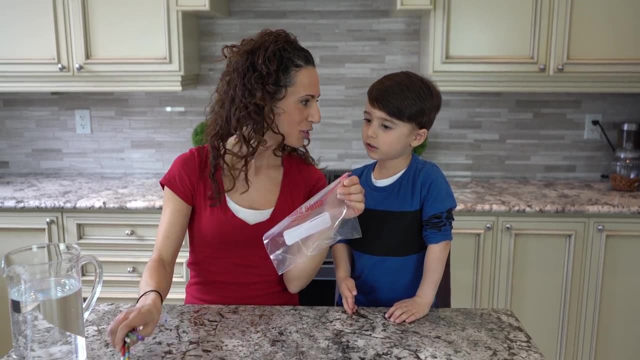 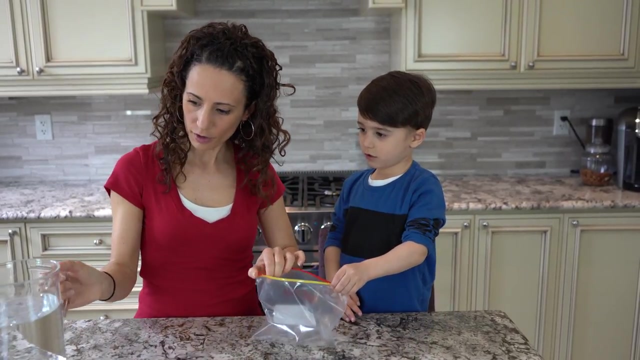 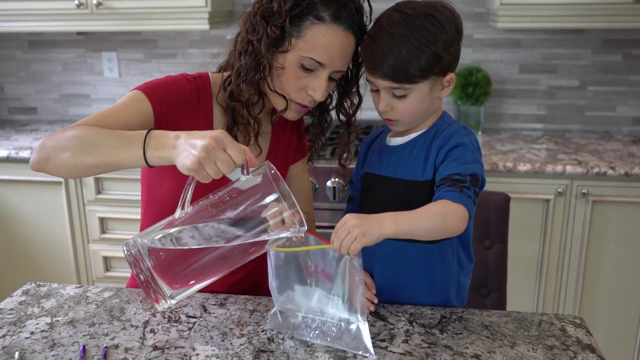 does my it pretty like my it. and now i watered mine. get ready to do. what sweet this is. a pot, that's cool. hold your hand on mine. that's cool. jelly, that's cool. show them, show. yeah. our third experiment is the plastic bag. and come to l isto работает, to understand how. 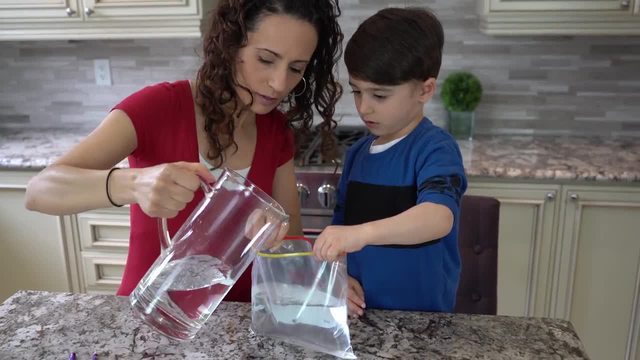 long you build up your Erin water. yeah, holding this際. so think I'm going to be water in a minute. experiment: we're going to fill it with water. yeah, hold it up, don't let it spill cold劉. Now we're going to put some food coloring so it looks even cool. 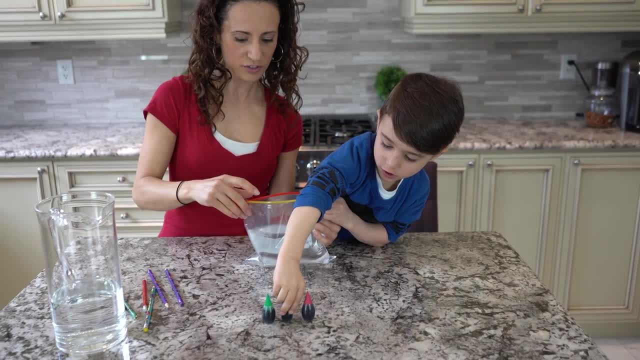 What color are you going to pick? Yeah, that's a good one. We got blue. Yeah, Okay, hold it here. still Hold it, Don't let go. I'm going to open it and then you put the drops in. 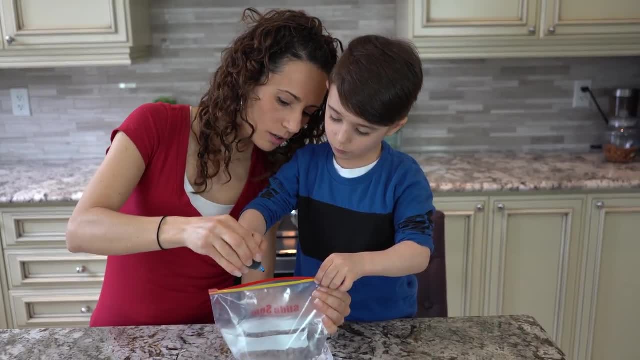 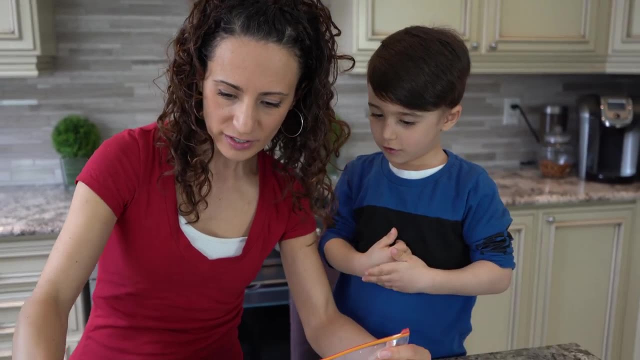 Okay, go, You put the drops. Ooh, that's a cool color. Wow, that's a nice color you picked. Okay, so we're going to get these pencils. now You ready? Here's your first one. Now we're going to poke a hole. 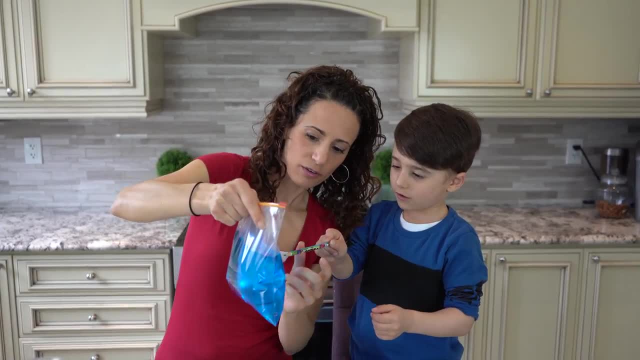 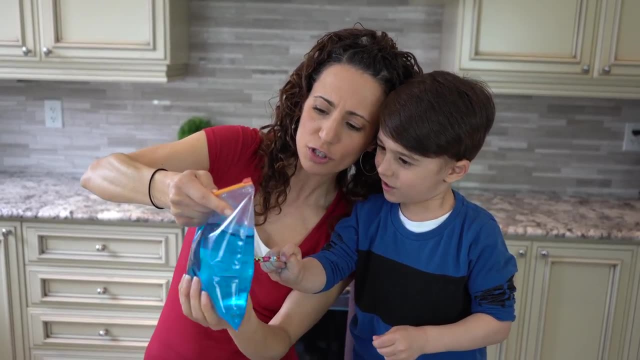 From one end of the bag and it's going to come out the other side. Okay, ready, Go in, Push, Push, Use your muscles. Go, push, push, Let go. Wow, It didn't leak. Okay, let me see how many more we can get in here. 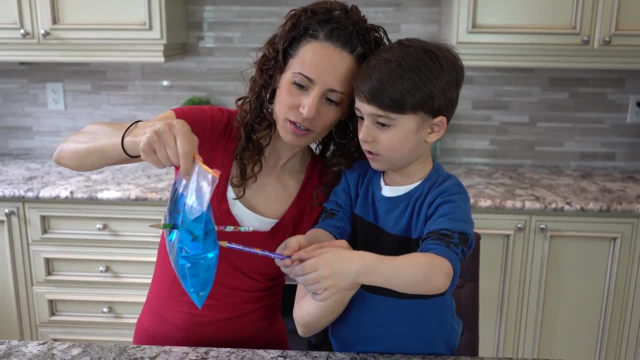 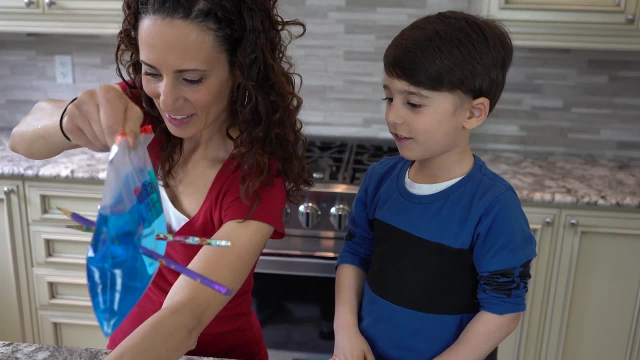 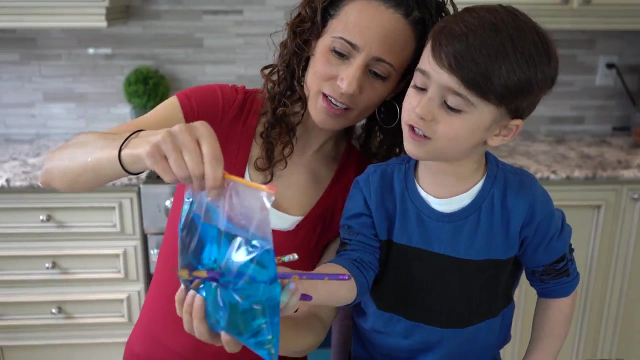 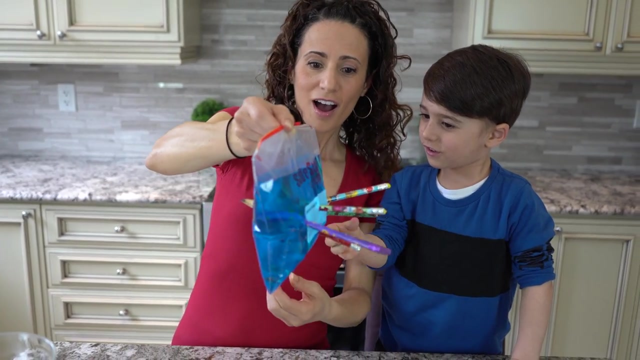 Okay, let's do this one now. Go, Push, Push, Push. There we go. We got two in. Okay, Number three: Okay, let's do this side. We got them all in. Yeah, Look at that. 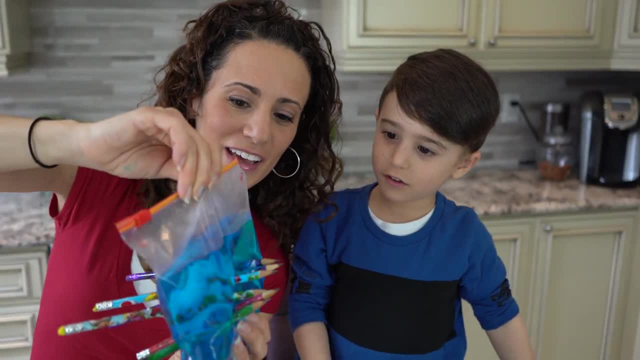 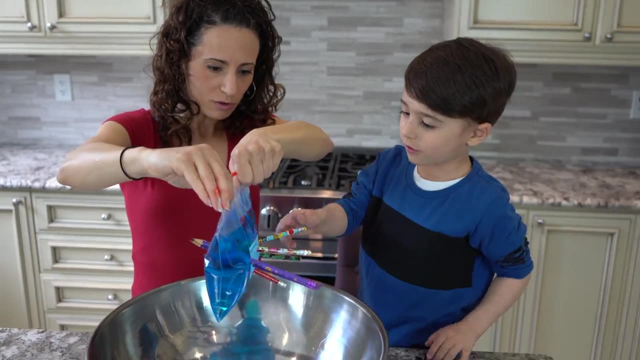 You can't take them out Ready. Okay, And now for the magic. What's the magic? We're going to take them all out and all the water is going to spill out. Pull them out. Pull them out. Which one first? 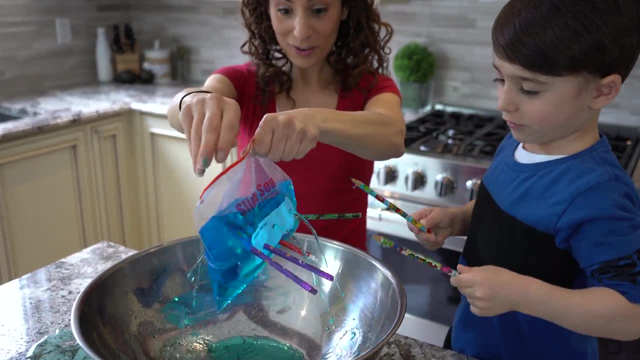 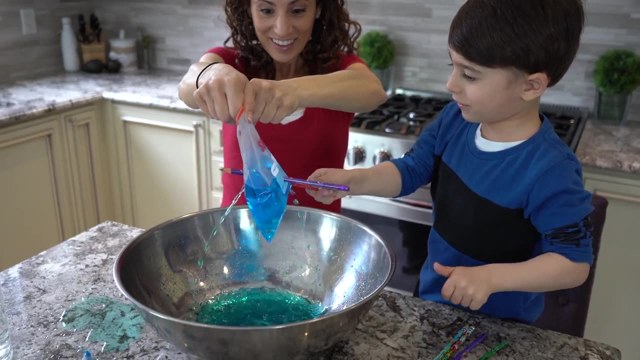 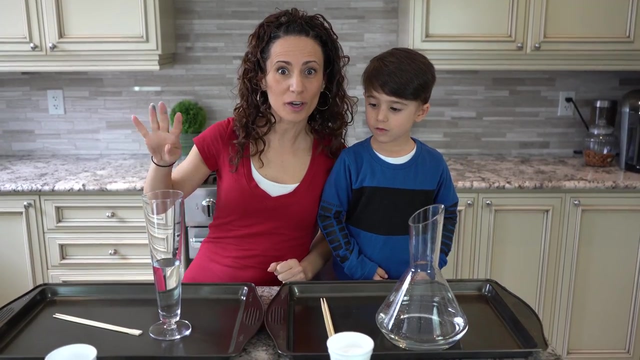 Let's go. Ah, Go, go, go, Keep going. Good job, That's fun. Go, Whoa, It's like a waterfall. Yeah, Whoa, It's a waterfall. Our fourth experiment is the vinegar and baking soda reaction experiment. 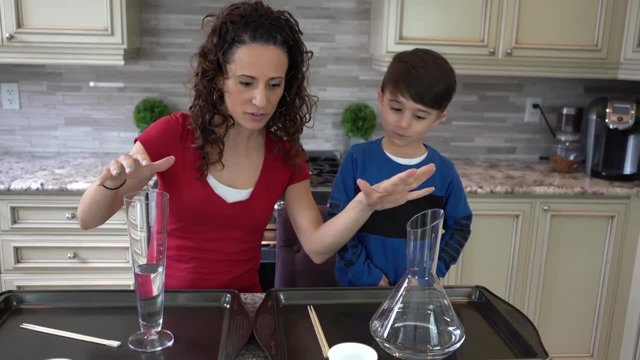 Ready? Yeah, Yeah, Okay. so we already have vinegar in the containers and we're going to add some food coloring. Yeah, and glitter, And glitter. You're right. Okay, what color are you going to pick for food coloring? 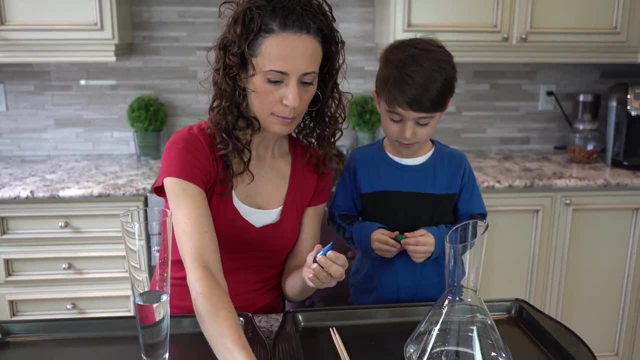 Um, green, You're going to pick green. Okay, you pick green, I'm going to pick red, I think. Okay, ready, Yeah, Do you want to help you open it Here? Put the drops in, Go. 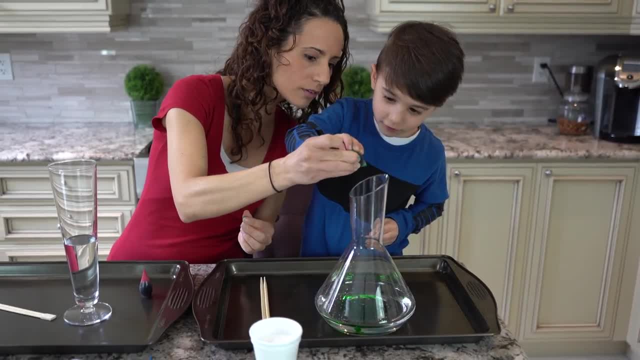 Squeeze Three, one, two. Is that enough Done? Okay, that's enough for you. Now I'm going to put. Look at that. Yeah, Isn't that cool? Okay, Mommy's going to put the red. 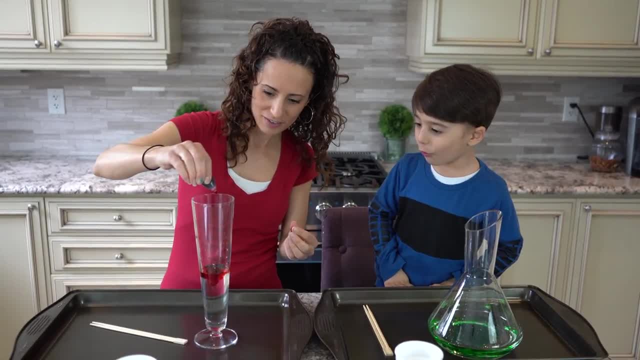 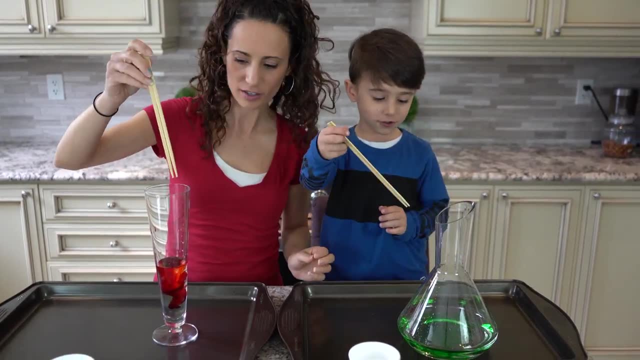 Whoa, Whoa, You're right, Yeah, Okay, Yeah, So let's stir. What do we call it? Stir, Stir, Ready, Agitate, Agitate, Go, Agitate, Agitate, Agitate. 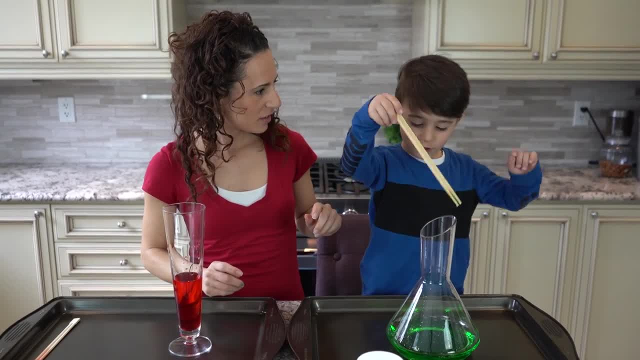 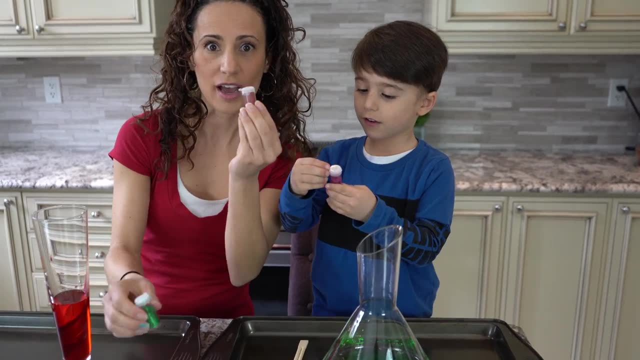 Stir it, Stir it, Stir, Stir. Yeah, Okay, it's all mixed, Mine's mixed. Mixed. Yeah, Mine's done. Do you want to add some cool glitter to it? Yeah, Okay, Do you want to pick a color? 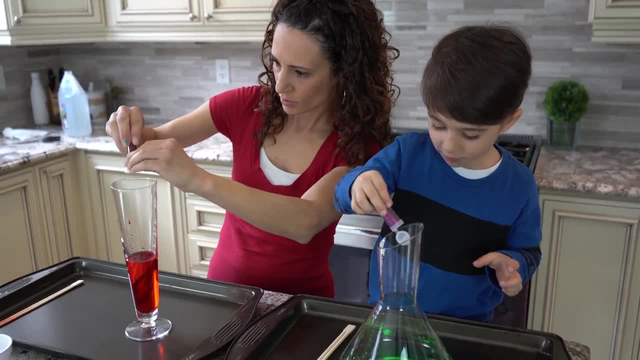 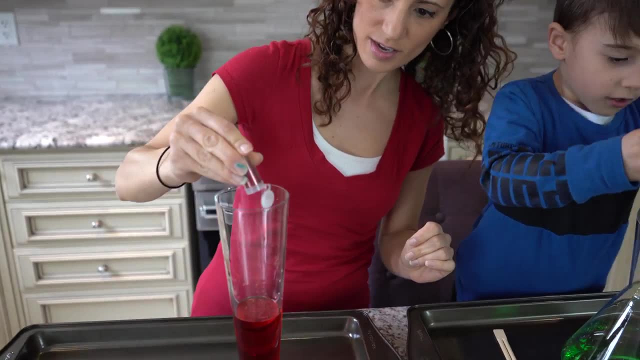 Um, I'm going to add pink, Pink. I'm going to add more red to mine. More red, Yep, I'm going to do pink. Okay, go Sprinkle it inside, Sprinkle Hard, Hard Yeah. 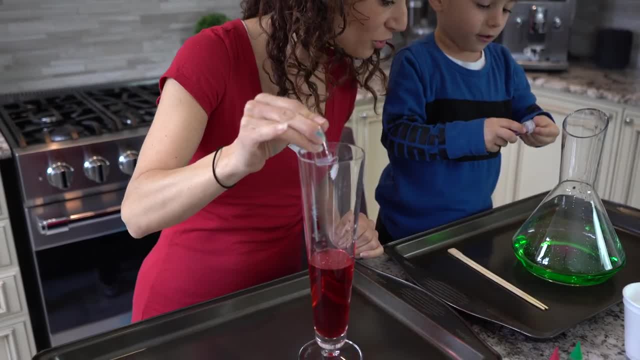 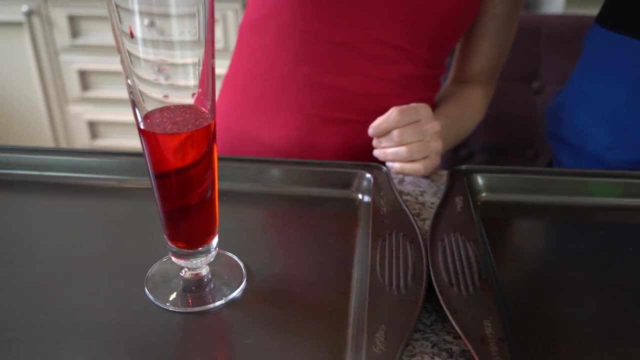 Look how sprinkly I'm going to do it like that. Oh, yours is really cool. actually, I like that. That's a good mixture. I want to stir. Yeah, Okay, go Agitate it, Stir, Agitate. 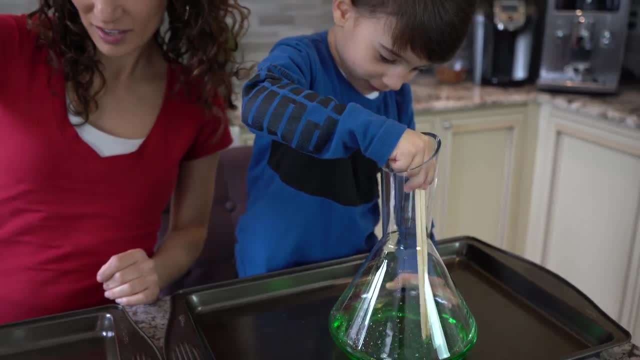 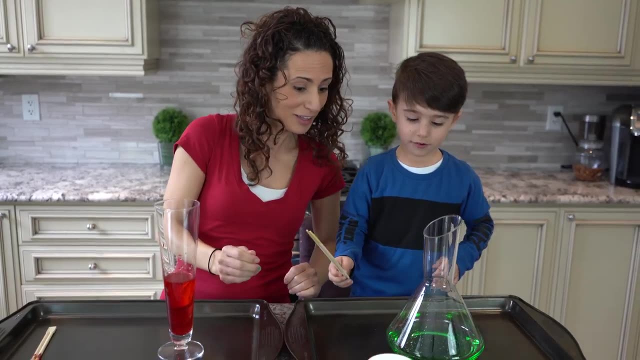 Agitate, Agitate, Agitate. Yeah, Stir it, Stir. Okay, So now. Well, mine looks pretty, It looks really good. So now we're going to add the baking soda. So when baking soda goes into vinegar, it's going to cause a. 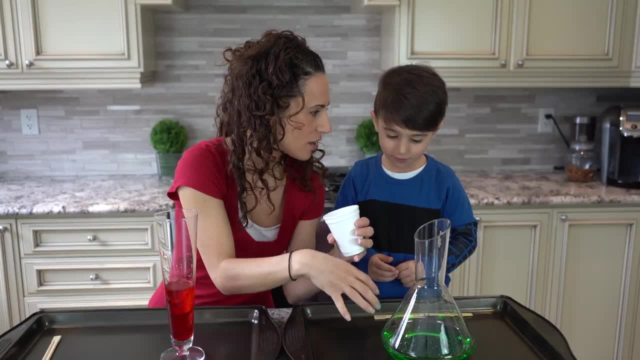 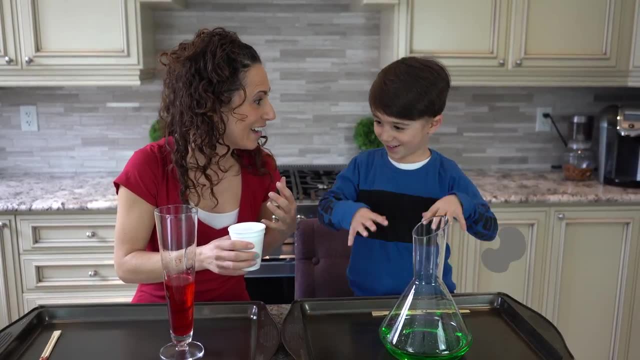 A, A, A, A A. A great reaction. What's going to happen? What do you think? Let's see Pour it in. What do you think, though, It's going to explode? You think so, With a volcano. 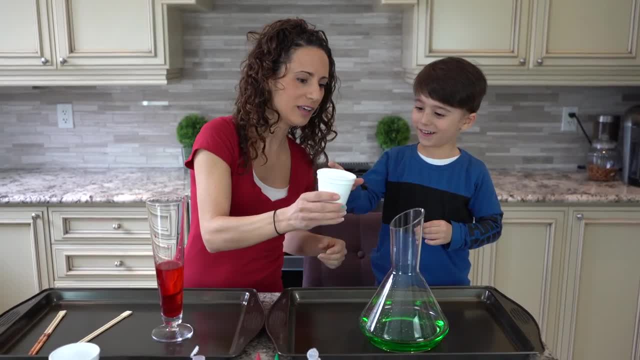 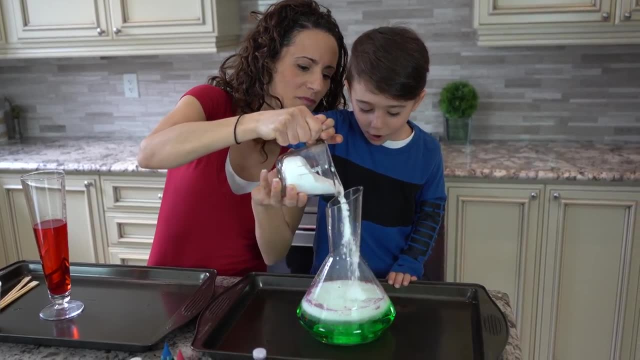 Okay, Are you going to pour it? Do it, Do it, You do it. Or you're going to pour it Ready, Okay, Okay, Here I'll help you. Ready, Ready. Let's see One, two, three. 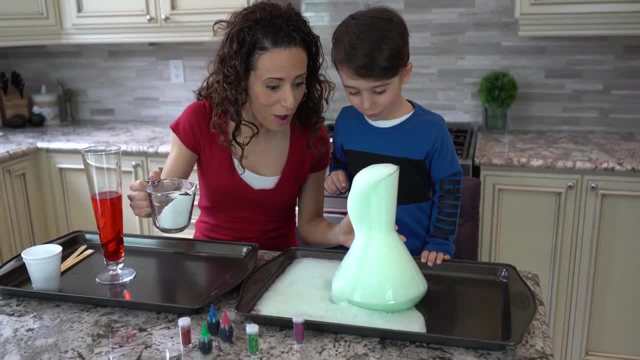 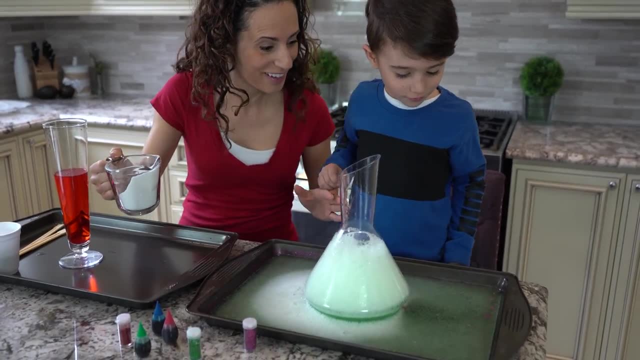 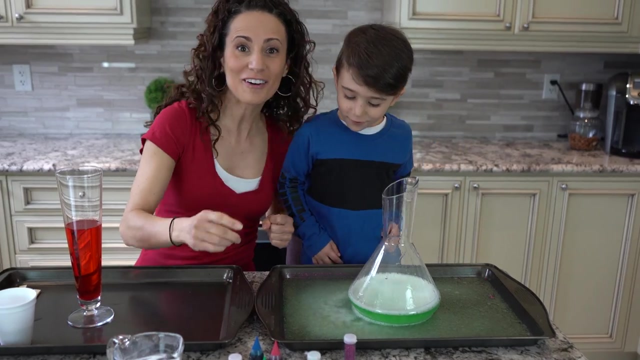 Go Go, Volcano Explode. Oh, Oh, my goodness, Volcano, That's so awesome. Luckily I destroyed the bottom. That's pretty cool. I love that, Mateo. That was cool. Oh look, it went all the way to here. 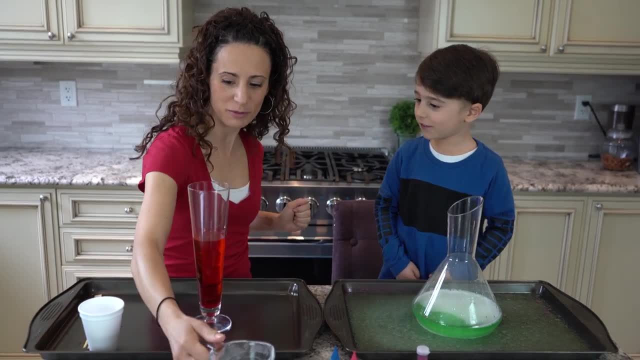 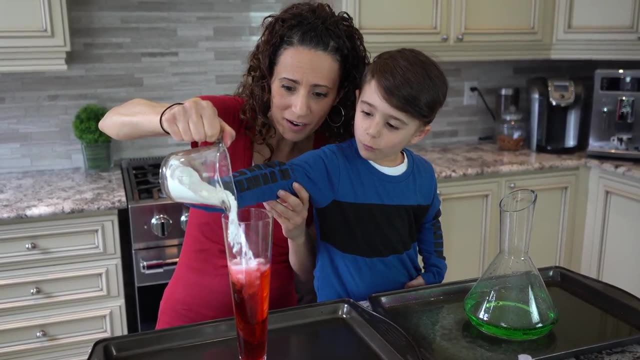 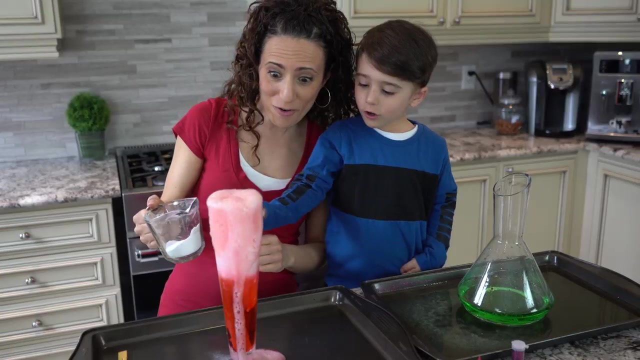 Okay, you want to do mine now. Let's see the red one Ready. Can you help me? Let's count down? Go One, two, three, go. Whoa, That's amazing, Cool Yeah, Volcano. 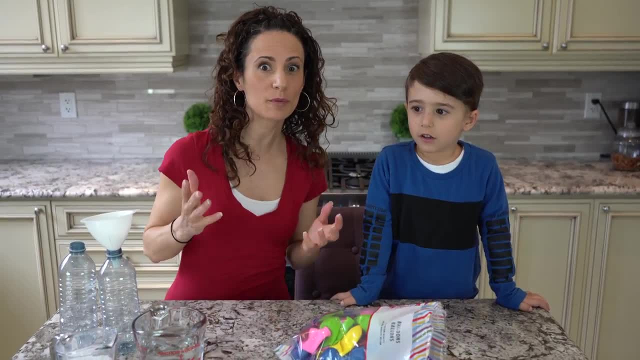 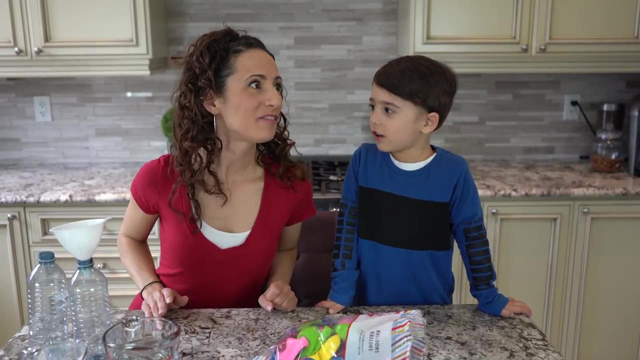 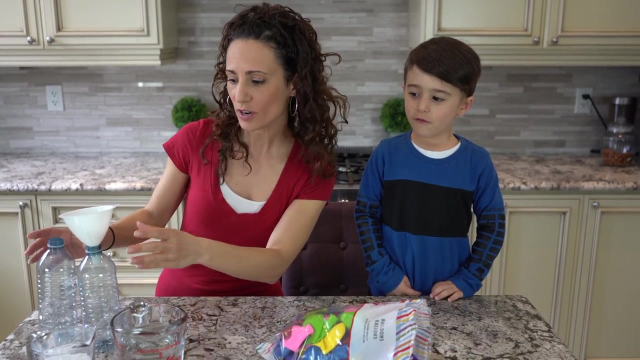 Yeah, Our fifth experiment is the balloon inflating experiment. A balloon inflating. One more time Balloon. Balloon Inflating, Inflating, Very good, Okay. so we're going to need some vinegar, some baking soda. 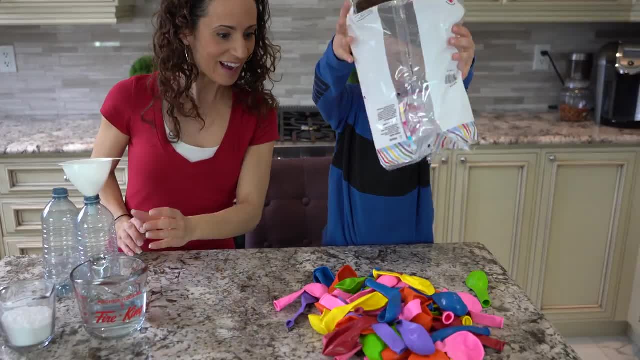 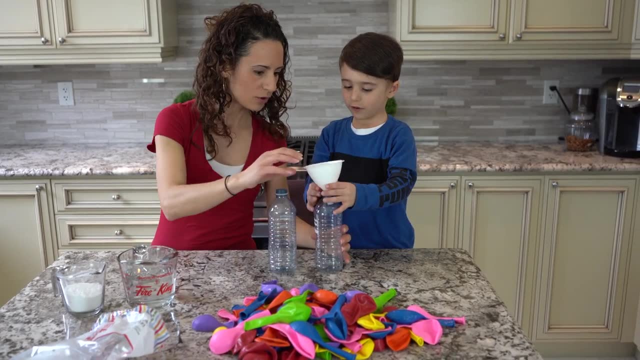 some water bottles and some balloons. Yeah, That's right, Lots of balloons, Good, Okay, so first we're going to hold the bottles. Let's start with the bottles. Can you hold them? Yeah, And hold the funnel for me, okay. 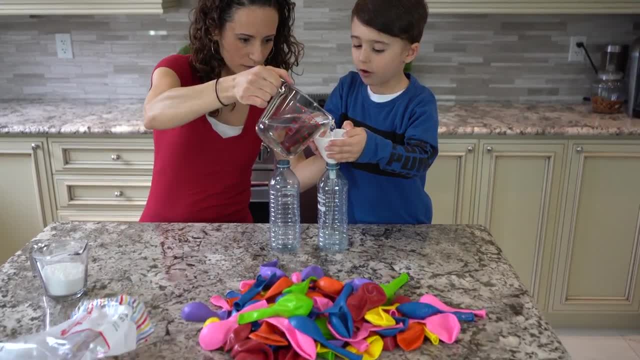 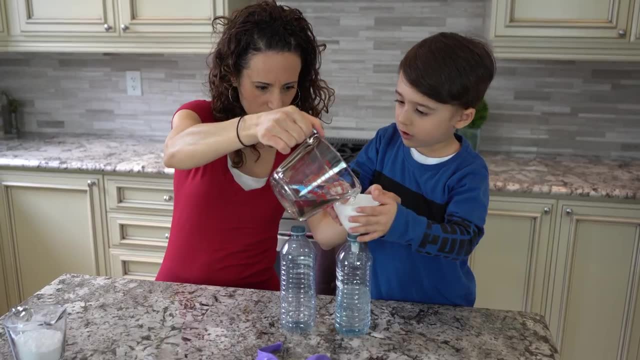 So we can pour the vinegar inside. Let's pour that in. Put it in the middle, Right in the middle, Then pour it up. You think that's enough? Yeah, A little bit more. Yeah, A little bit. Which balloon would you like to pick? 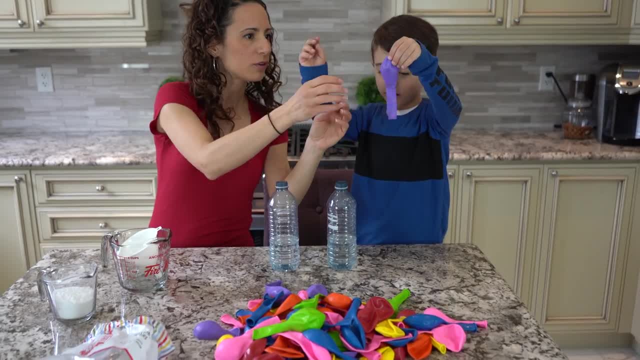 I want to pick the purple one. The purple one, Okay, And I'm going to pick. I think I'm going to pick the red one. What do you think? Good Yeah, We're going to fill the balloon with baking soda.